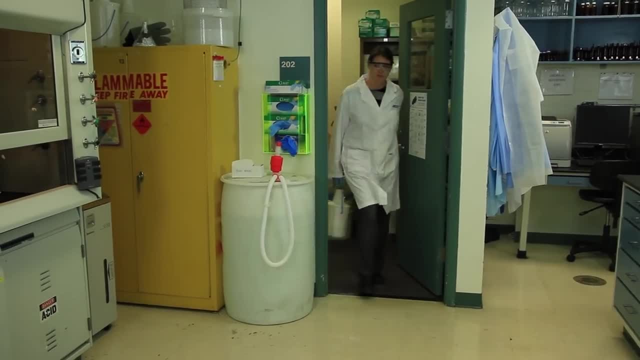 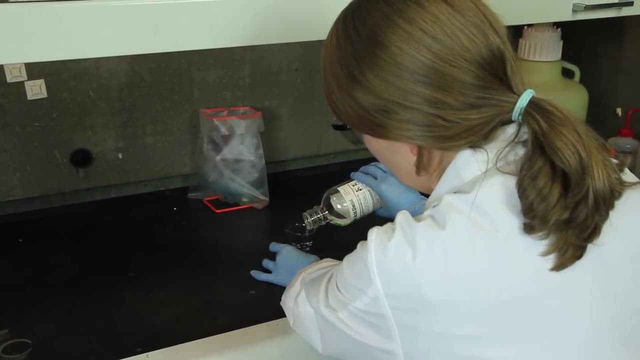 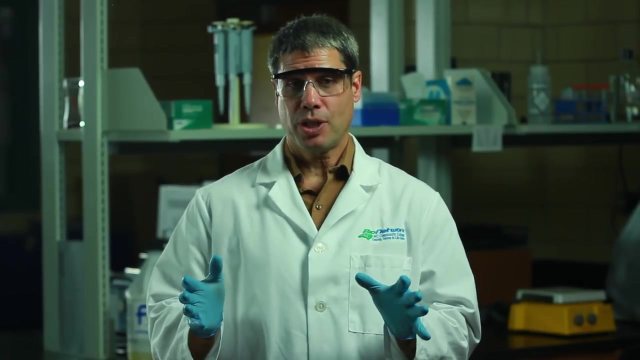 Never remove chemicals from the lab. Use a break-resistant secondary container to transport chemicals between lab spaces. Chemicals must be handled safely in order to avoid skin, eye or inhalation exposure. First, let's talk about protecting your eyes, As we mentioned. 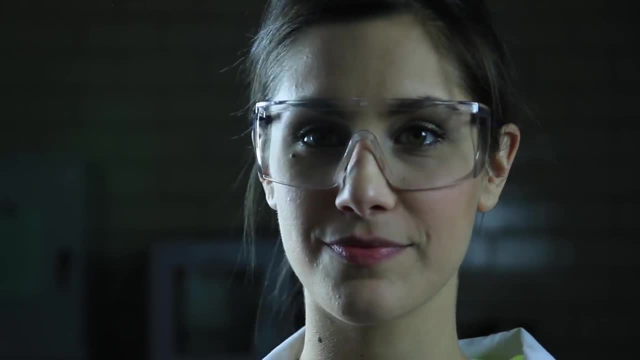 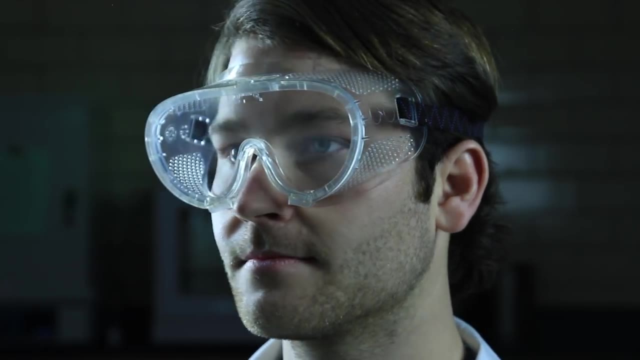 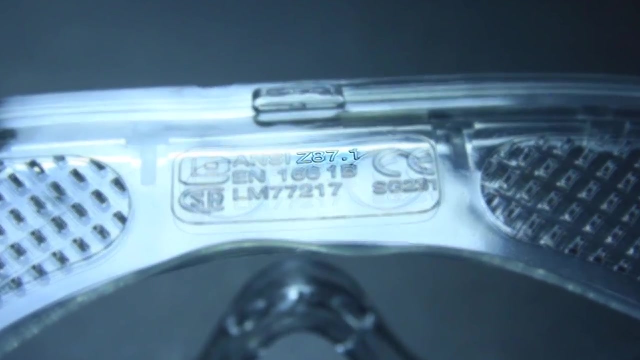 in our lesson about PPE. safety glasses with side shields offer some protection, but they won't help you when working with a potential splash hazard. Splash goggles are more effective at protecting your eyes. Chemical splash goggles should be marked with the code Z87.1.. This 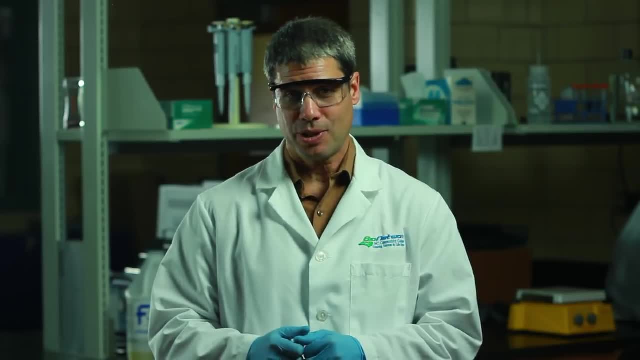 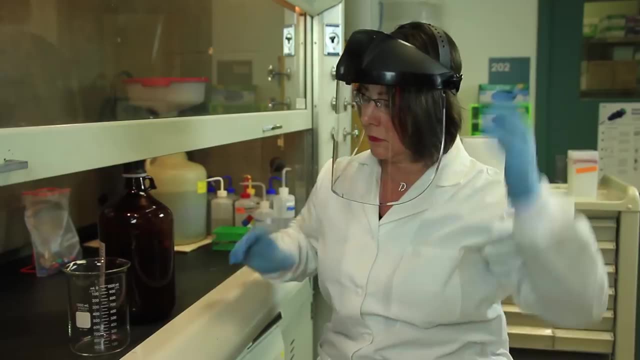 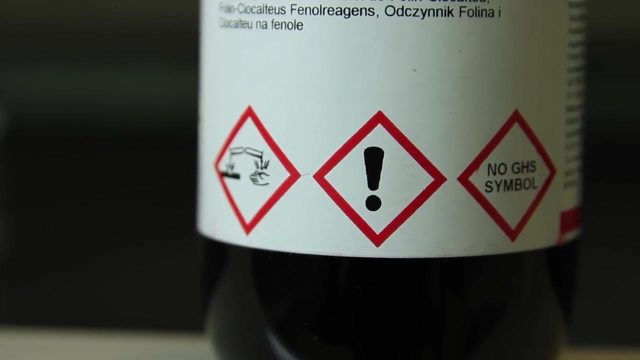 code indicates compliance with American National Standards Institute. Prescription glasses don't offer adequate eye protection. Wear safety glasses, Goggles or a full face shield over your prescription glasses. Corrosive chemicals will harm you if they splash or come into contact with your skin. A lab coat and gloves will help protect. 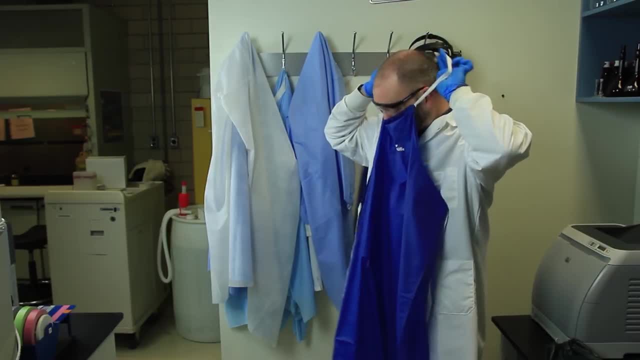 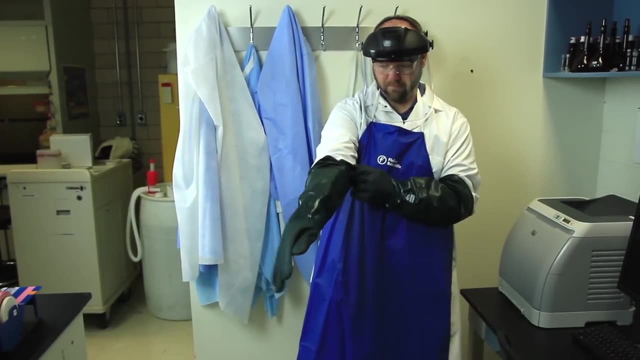 your skin to a degree, but a full-length chemical-resistant lab apron is the best choice when working with splash hazards. If you're working with an especially corrosive chemical, use full arm-length rubber gloves instead of the typical nitrile gloves. 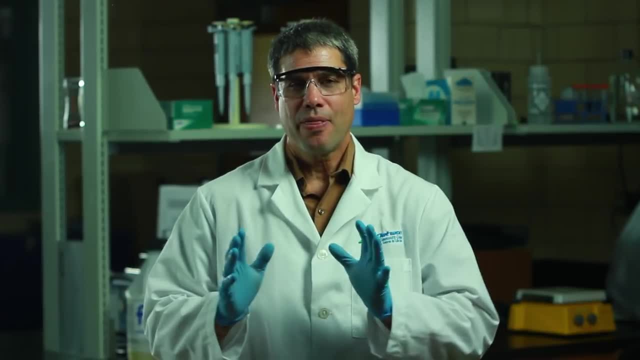 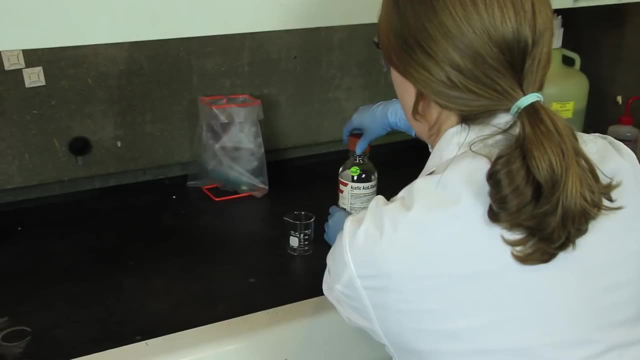 Some chemicals in the lab can harm you without even touching you. That's why it's important to be aware of inhalation exposure. Never smell chemicals, Always work with toxic chemicals under a fume hood And keep containers closed tightly if you're not using them. If a large 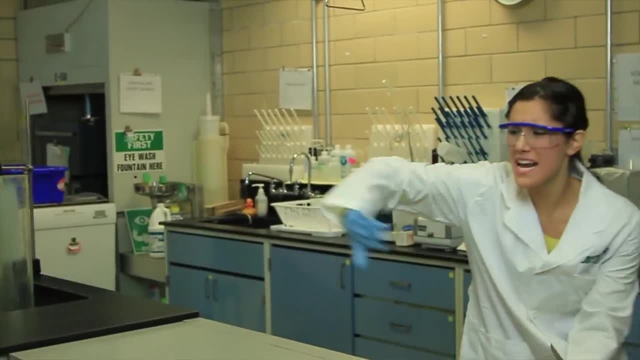 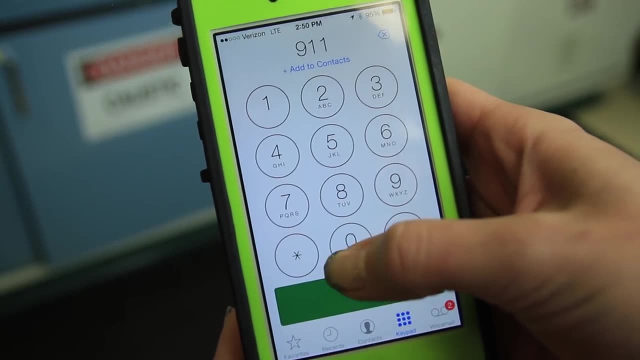 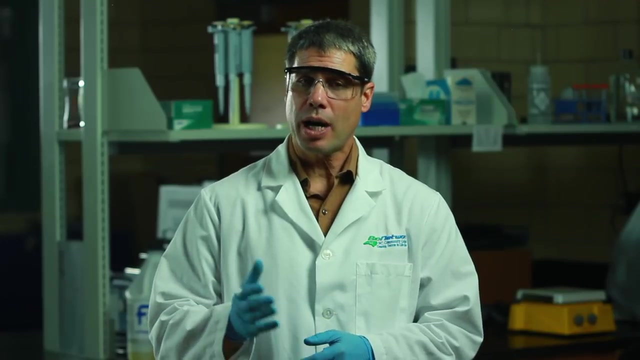 chemical spill occurs, evacuate, seal off the lab and notify the authorities. Large spills can produce excessive vapors and have to be cleaned by qualified personnel. Don't re-enter the lab until your supervisor gives you the all-clear. Flammable chemicals require special handling techniques. First, always know the flammability. 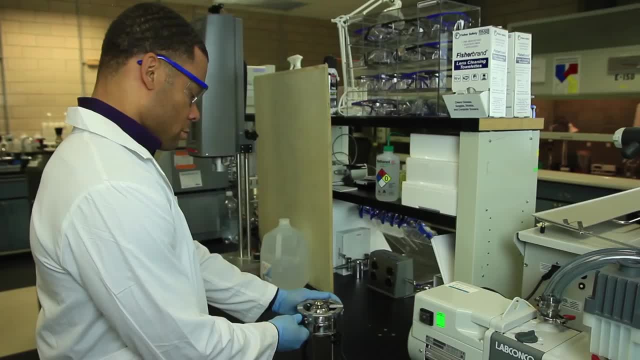 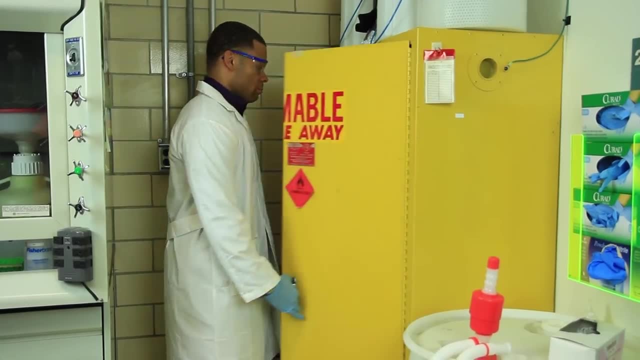 and explosive potential for each chemical you're working with. Keep flammables away from all ignition sources such as Bunsen burners or hot plagues. Store flammable chemicals in a dedicated and grounded storage cabinet When you're finished working in the lab properly.